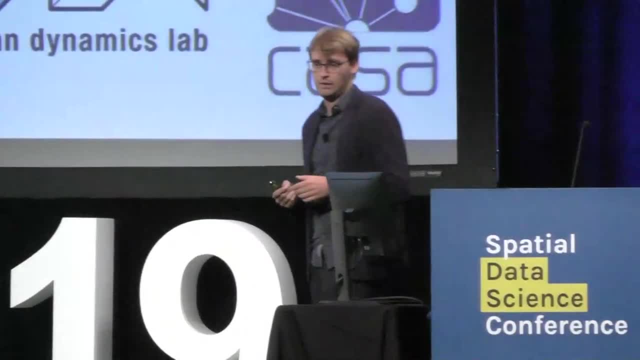 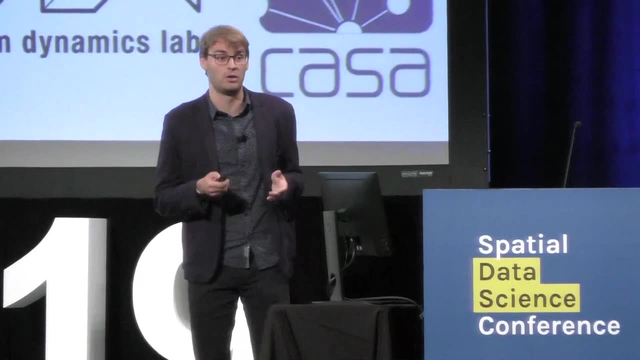 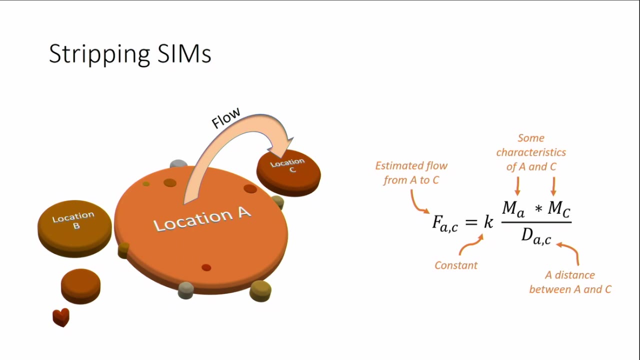 it. Okay, it's not me, Great, Okay. So I'm Martin Vanhoof. I'm going to talk a bit about spatial interaction models. There's a whole family of these models out there, but basically, if you reduce them to their essence, they're about predicting flows or interactions between. 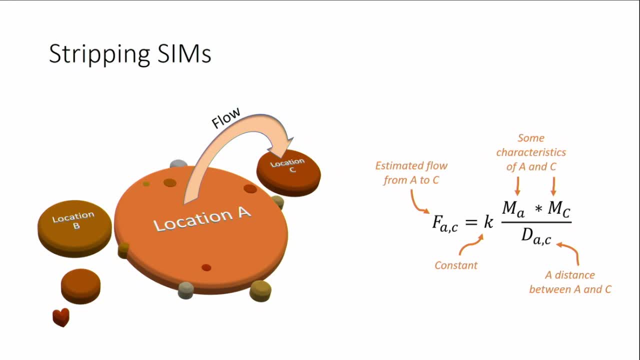 different areas, based on the characteristics of these areas and some distance measure. Now this might seem very simple, right, But in the past these models have been very useful for, for example, retail locations or urban planning- One of the interesting bits about CASA. 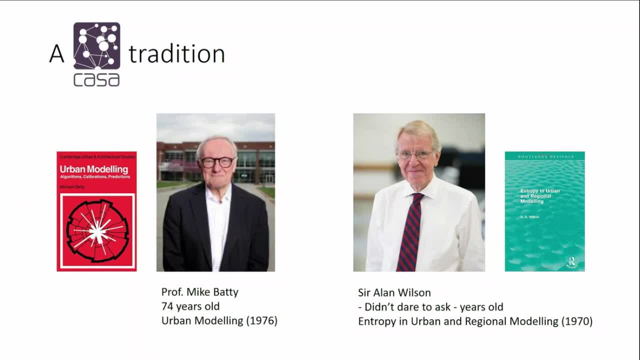 the place where I work that's been promoted very well already here is that the people who popularized these models are still working there. They popularized these models in the 60s and 70s And this makes well. actually it makes you wonder why they're still not retired. But it also makes you wonder. 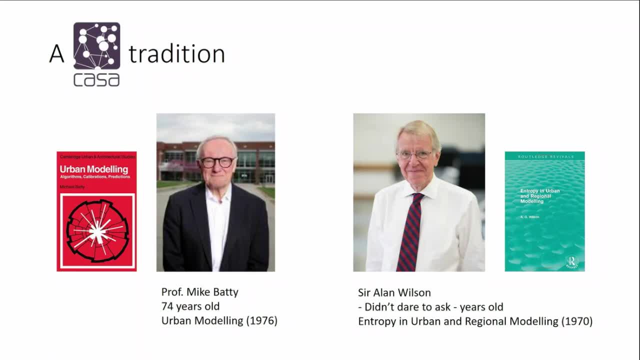 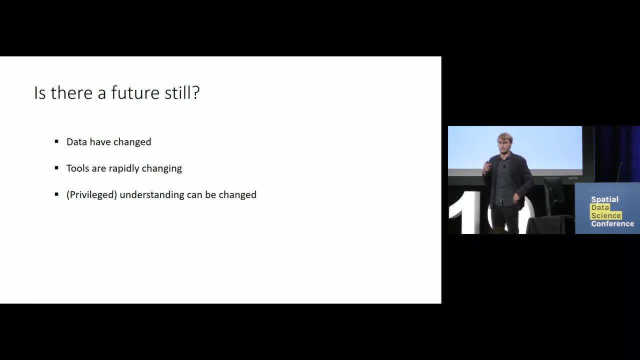 to which degree, why and how these models would still be relevant today. So let me try and raise three points to you today as to why I think these models are still relevant. I know I'm preaching a bit to the choir here, but one of the of the 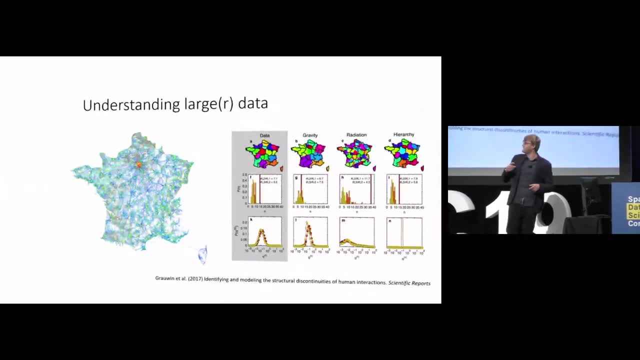 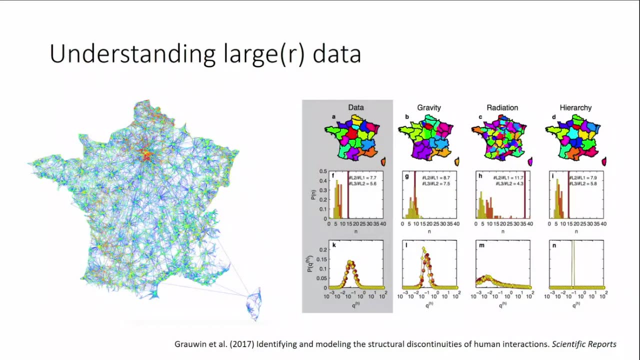 the obvious things is that the data is different today, right, What we see is that, compared to before, where these spatial interaction models would be used to fill in missing data that was not collected by surveys or census, nowadays there's this, this tendency towards. 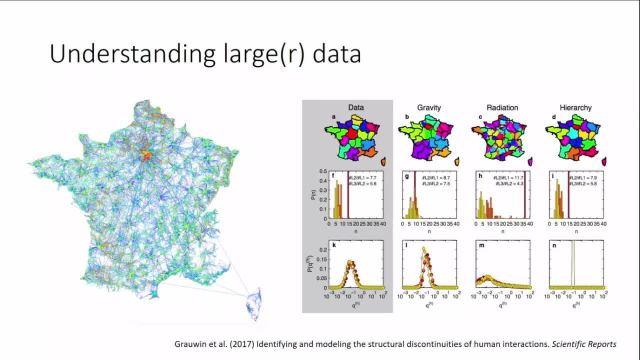 using the spatial interaction models to understand large data sets. For example, this is one of the works I did with MIT and NYU, trying to use spatial interaction models to better understand the calling patterns in France between cities, actually between locations. So basically, what we did is we we used a lot of spatial interaction models to see whether 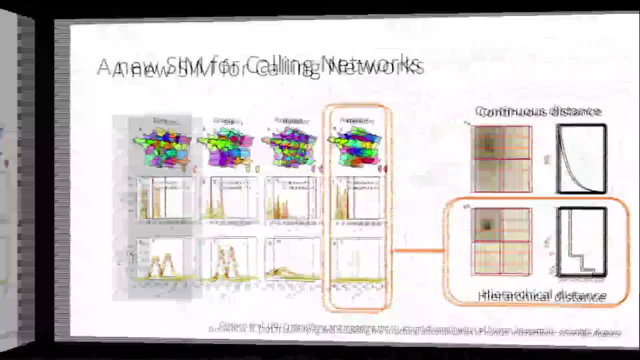 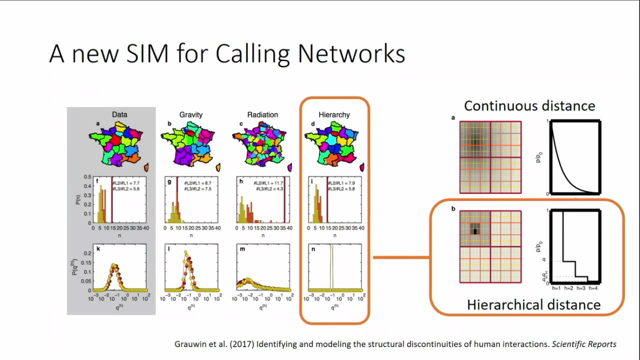 we could capture the patterns in these calling data And what we found is that actually calling in France, and also in other cities and other countries in the world, is not necessarily dependent on the continuous distance, but rather on the hierarchical distance, And you do know this effect from your own life. It means that you're more likely to call to a 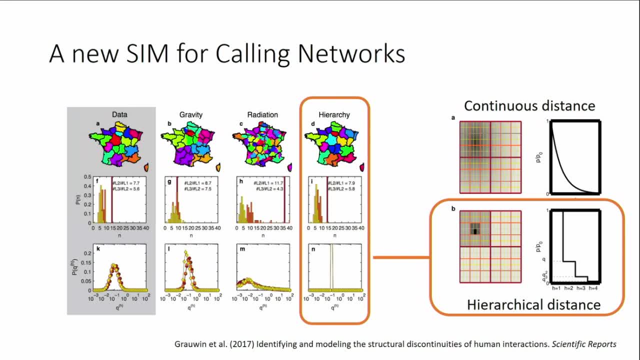 regional center which is a bit further away, or even a national center which is really far away than you're likely to call to a similar center. So the neighbors you never speak to really. So this effect is actually captured by the spatial interaction models in this paper. If you're interested, just read it or come. 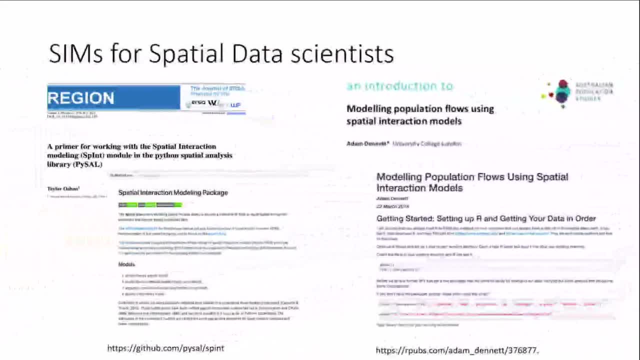 to me afterwards. Another thing that I think is adding to the relevance of spatial interaction models today is that we are now having the tools and the technologies to actually run these models, Or at least for a lot of people to run these models And what you see in the academic world. 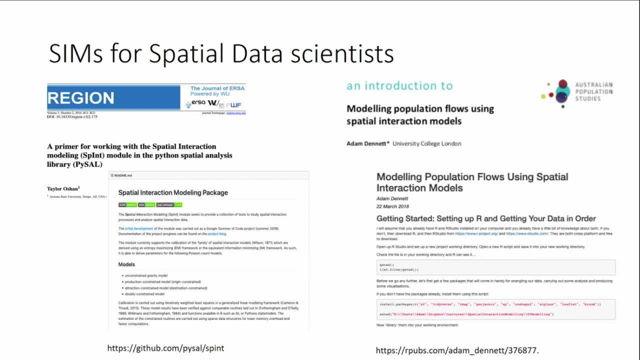 more and more researchers are starting to publish these tools, these frameworks, to accompany their own research. For example, Taylor-Ossian has this great Python library called spint, which actually allows you to do spatial interaction models. Now, opening up these kinds of tools and frameworks, I 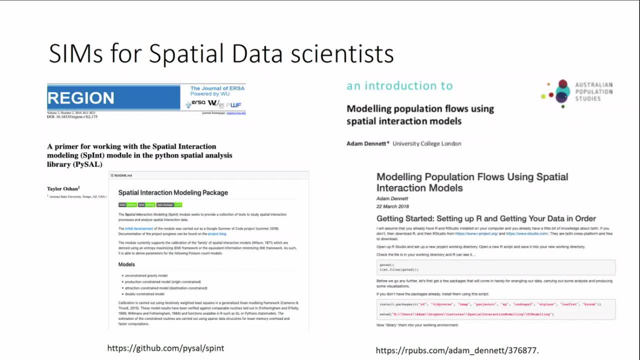 think is 100% laudable, but I have to admit that I'm not entirely convinced this is the best way to go. reason that these spatial interaction models are actually rather complex. They require quite some user decisions on the parameters, the performance indicators. 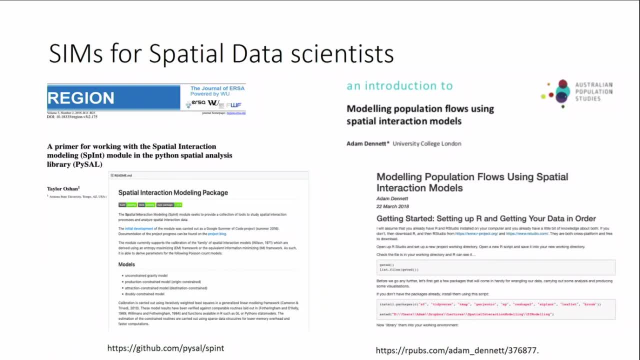 and the statistics need quite some interpretation from experts, and if you get them into these libraries, you automatically end up in this kind of oh, I use this line of code and I set the default parameters and ta-da. We've all been doing this, me included, but there's a danger that we're not simplifying the 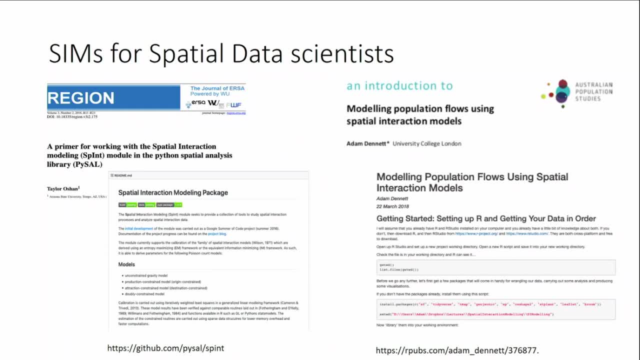 models or neglecting our understanding of the models. So, fairly spoken, I think academics like me, we should try to reach out more and try to get this educational, sometimes criticism on how these models are being used by normal spatial data scientists, and elaborate much more on. 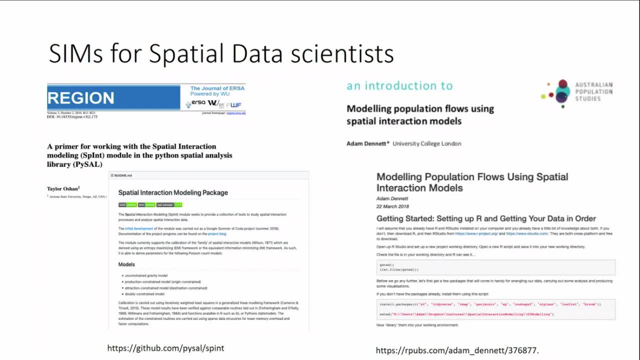 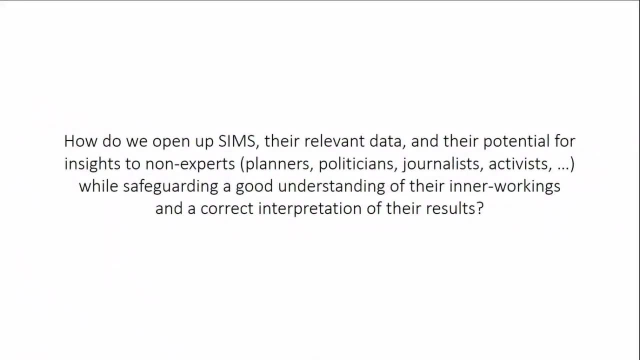 this. We don't do this very well at the moment, but this is certainly something we can improve on in the future. A final point I'd like to raise is- and this is some of the work we're doing at CASA at the moment. some of the work: 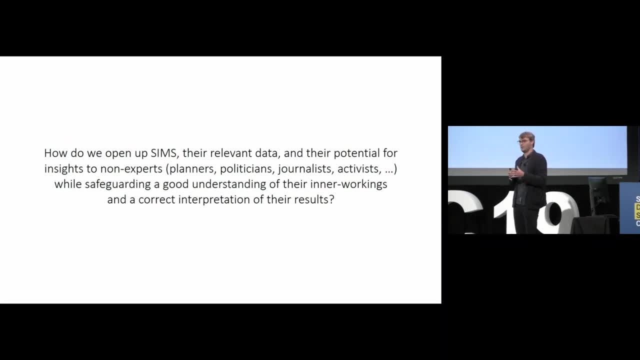 I'm working on is that I think we could even open up this kind of spatial interaction model, these kind of models compared with data and interpretation, to a much wider audience than just spatial data scientists and other researchers. This is essentially what we're trying to do in this project called.